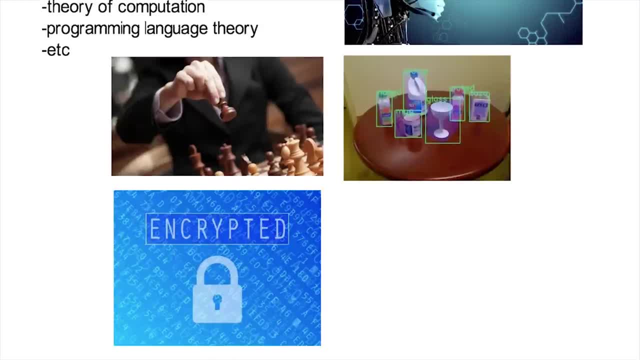 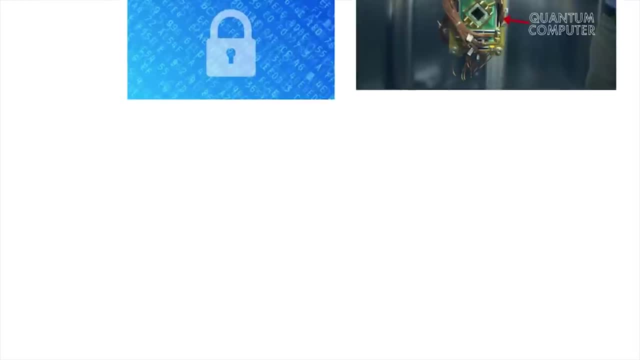 with data security and cryptography, so sense of information remains secure. Or computer scientists are even needed for quantum algorithms, when it comes to quantum computing, which is not a huge field yet, but is another example Then. So software engineering is where you use many computer science topics, such as algorithms. 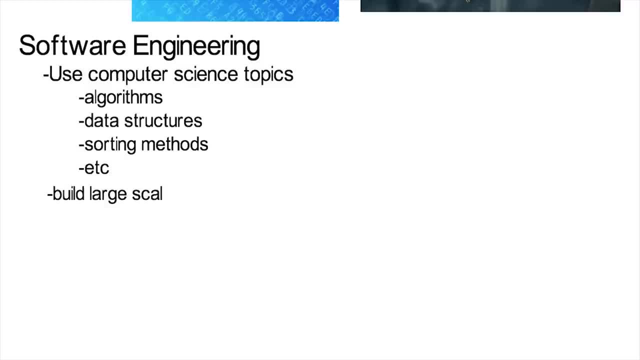 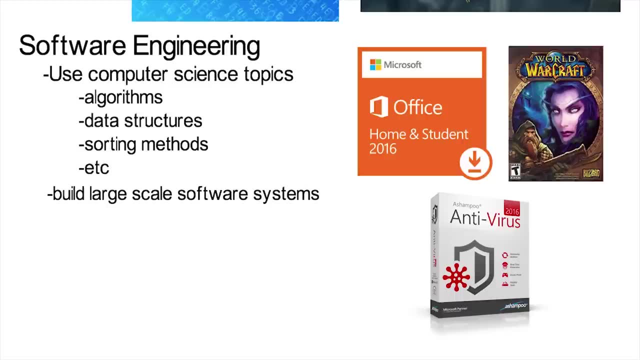 data structures, sorting methods and so on to build large scale systems. They are the ones who are needed when products like Microsoft Office, World of Warcraft or new anti-virus software are going to be made. These things can contain millions of lines of code. it's not feasible for just one person. 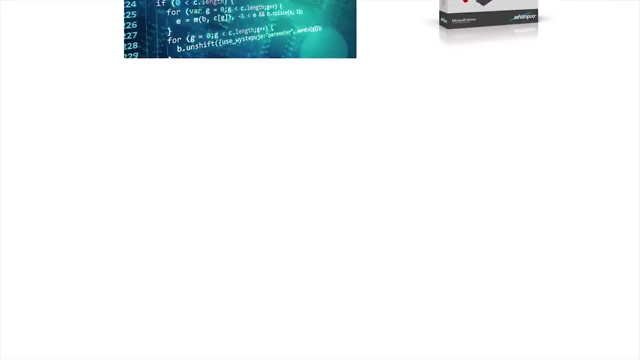 and you can't have a bunch of programmers just dive in. There's more structure to it. They have to understand all the requirements for a project plan, the life cycle of the software, figure out how to implement everything, and then they have to figure out how to implement. 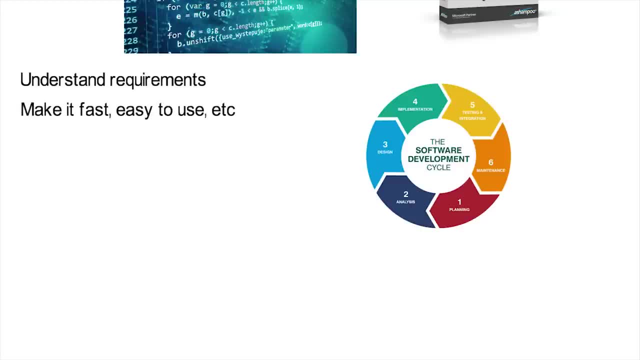 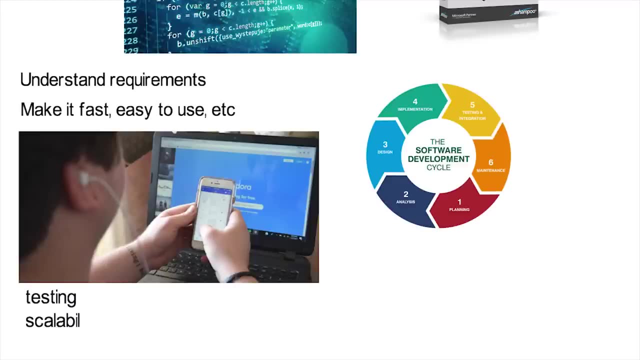 everything like it might need to be fast, super easy to use, etc. They think of who will be using the final product, like if it will be other engineers or just an average person. They have to do testing, think about scalability and so on. 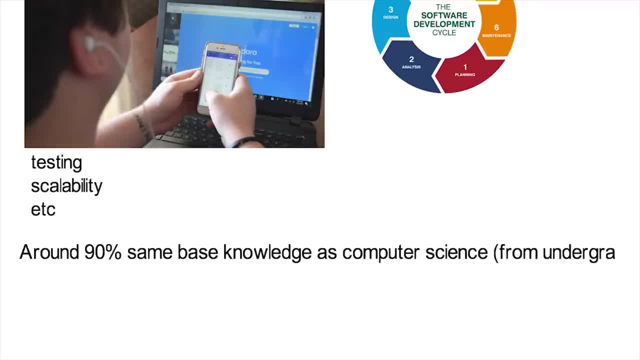 A software engineer has like 90% the same base knowledge as a computer scientist, except they aren't really concerned with discovering an even faster method of sorting a list of items. They'll use sorting algorithms that have already been discovered, likely by a computer scientist, to make their code and system work efficiently. 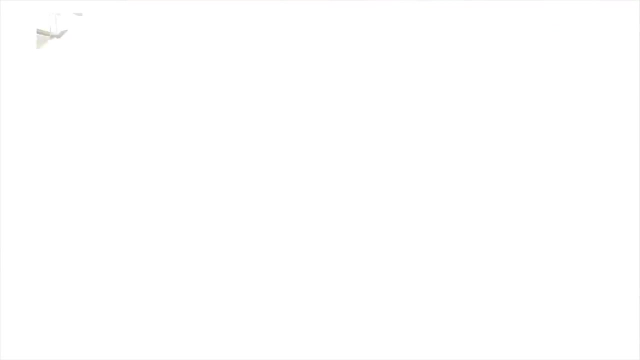 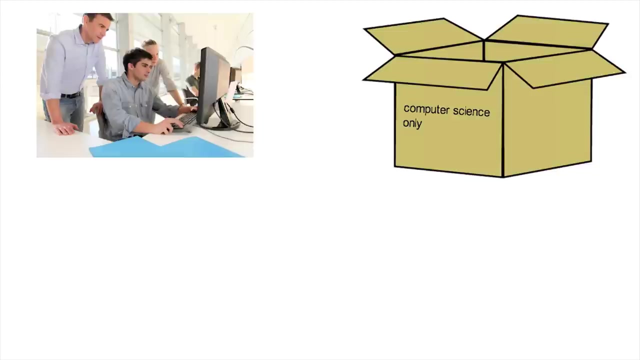 Now these are how you can define both fields, but if you look at reality and actual jobs, you won't see people divided so neatly. It won't be like if you majored in computer science you were put into this box of careers in AI, cryptography, algorithm design and so on, where no software engineers 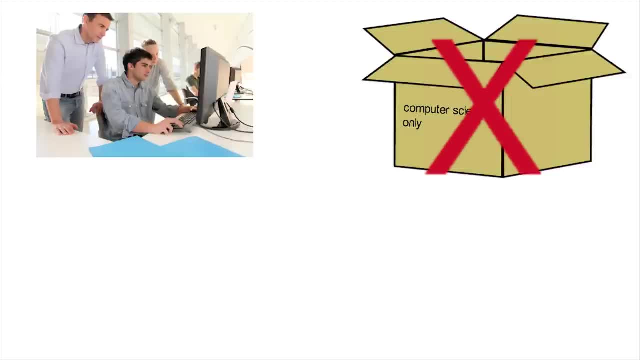 can enter and you'll never leave. That's not at all how it works. People in these two disciplines are totally mixed. The roles are essentially interchangeable today, and most job listings will say something like computer science or equivalent discipline required, which usually means something like software or computer engineering. 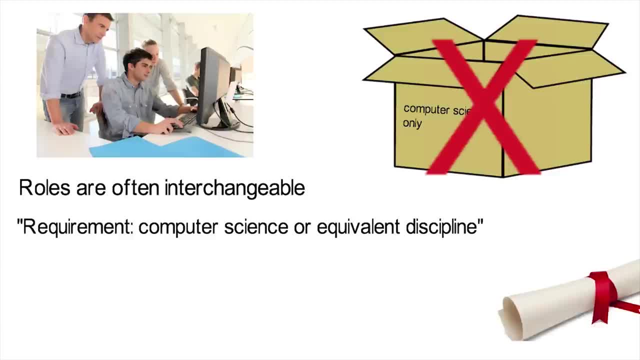 I also said that many computer science jobs are in research, but those typically require a masters or PhD And because most people don't do that, a majority of computer science majors end up in software engineering jobs. Most of your friends who graduate in computer 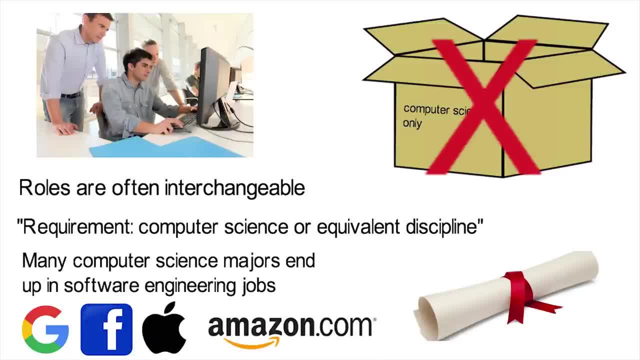 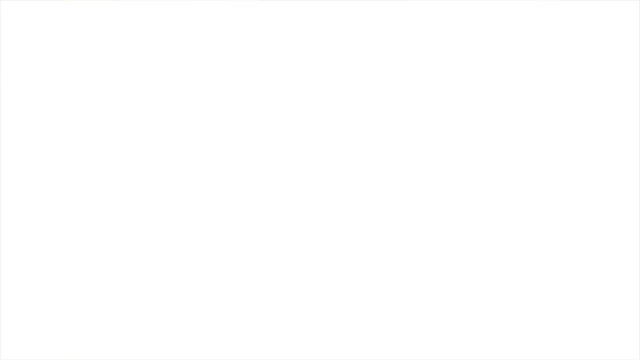 science and go off to Google, Facebook, Apple, Amazon, etc. are technically working in software engineering or software developer roles, building those large scale systems. Now, even though they have different definitions, when it comes to the college curriculum, they are extremely similar, So let's take a quick look. 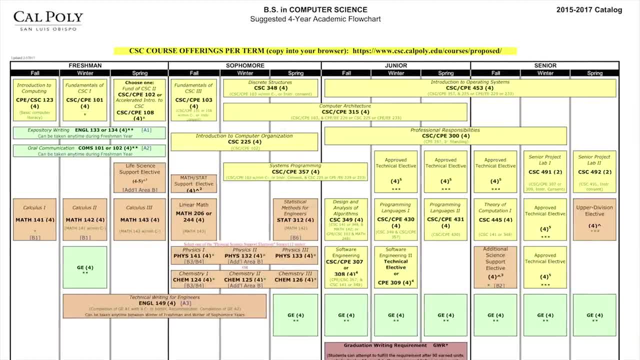 Here's the computer science role. This is the curriculum for my school, Cal Poly, San Luis Obispo, but note everywhere it is a little different. For now let's just look at these classes in yellow. as these are the major classes, I'm going to sweep through them first and then go into detail on a few. 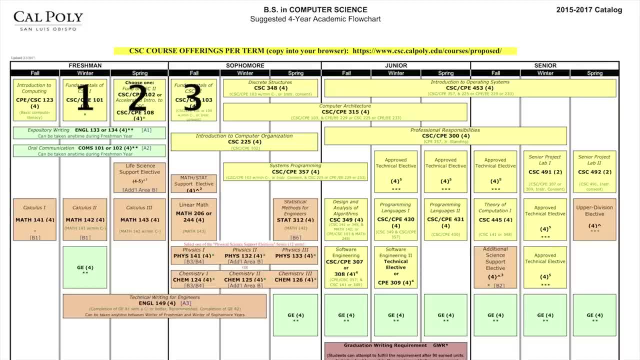 of them. afterwards They take these three programming courses that teach a lot of the basics. They take discrete math, this more computer hardware focused class, systems programming, which goes into more detail in the C programming language, algorithm design, which is very important in the programing language. This course is more about systems safety. code of ethics, intellectual. 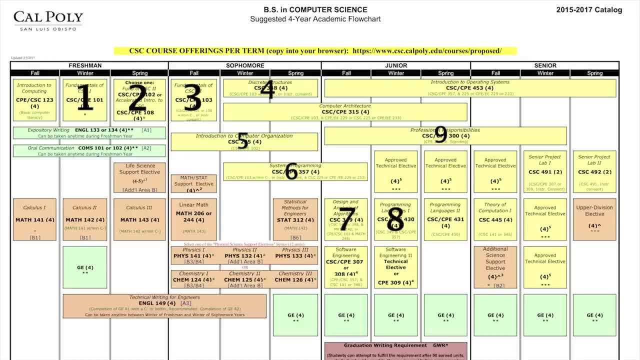 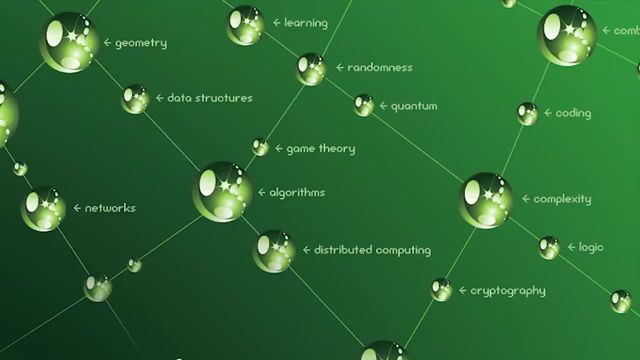 property and so on. These nine classes I just listed are all taken by software engineers as well. So you hear how computer science is more geared towards theory, math algorithms and so on. Yet software engineers have to take discrete math algorithms, and way more, Even if they. 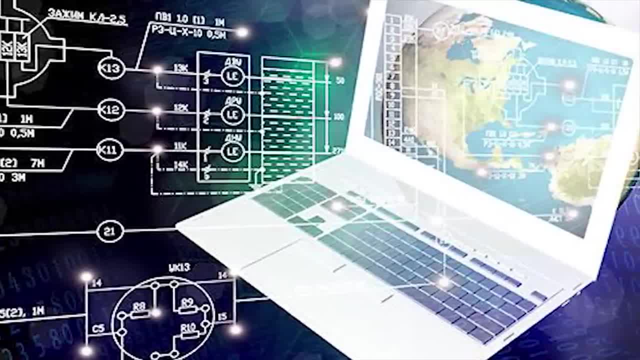 don't do as much research work later in their career. software engineers simply need all that computer science information still to work on their various projects. So even if they don't have as much research work later in their career, software engineers simply need all that computer science information still to work on their various programs. 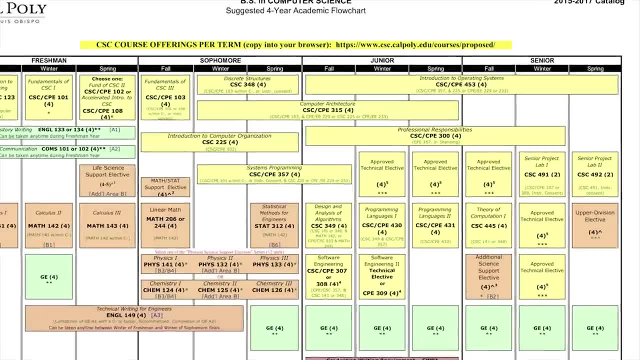 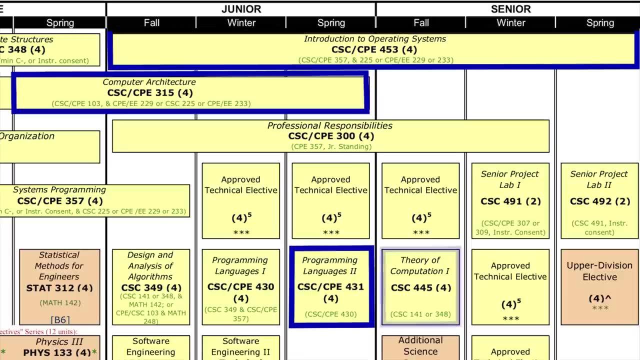 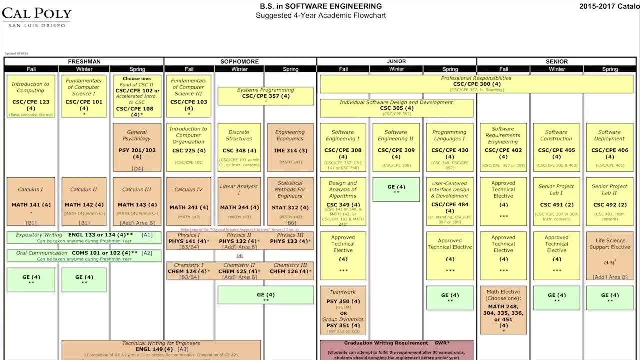 on their various projects. the remaining four classes are what software engineers are not required to take, those being computer architecture, operating systems, a second programming languages course and theory of computation, and of course this is not counting electives. if we go to the software engineering curriculum, those same nine classes come up, like i said, which leaves four. 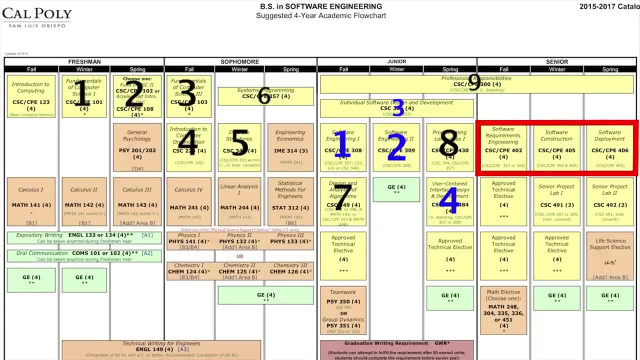 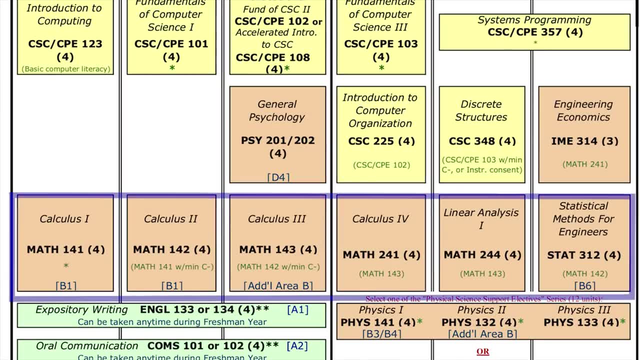 classes unique to software engineers. i'm not counting these three because these are kind of like another senior project class. i'll talk about these all very soon, but first, if you look at the math classes they take, you'll notice it's pretty much the exact same as the one computer scientists. 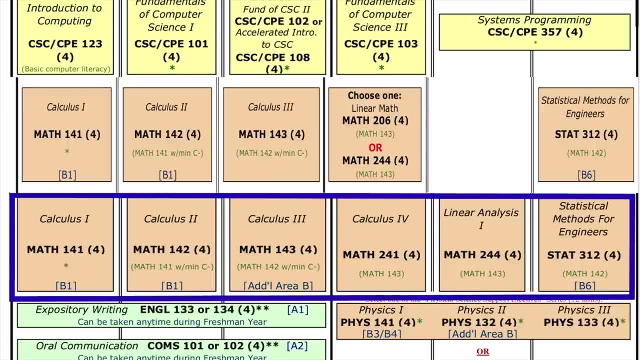 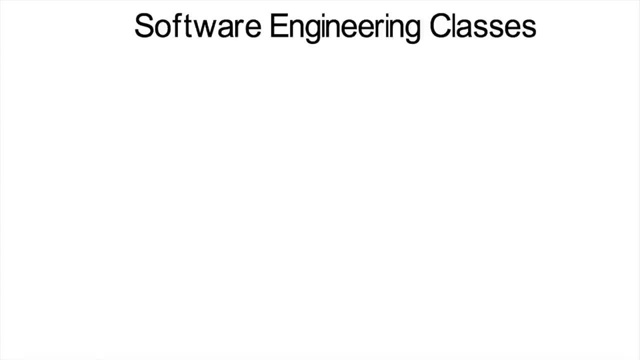 take, except computer science majors, at least at my school, are not required to take our calculus 4 or multi-variable calculus. now let's go back and i'll explain a little more about those classes unique to software engineers. but just as an overview, the software engineering specific classes. 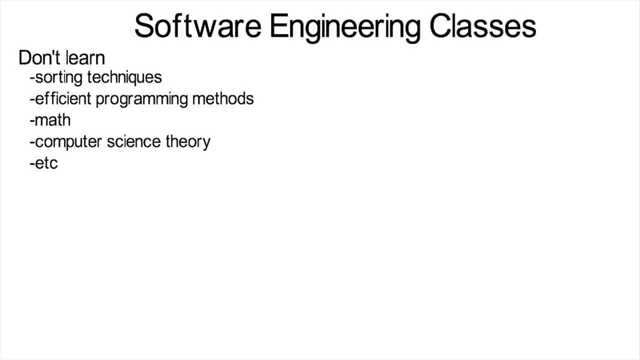 are not about learning new sorting techniques or more efficient programming methods or any more math theory or anything like that. they're not about learning new sorting techniques or more efficient programming methods or any more math theory or anything like that. they're not about learning new sorting techniques or anything like that. they're about how to plan out your project work as a team. 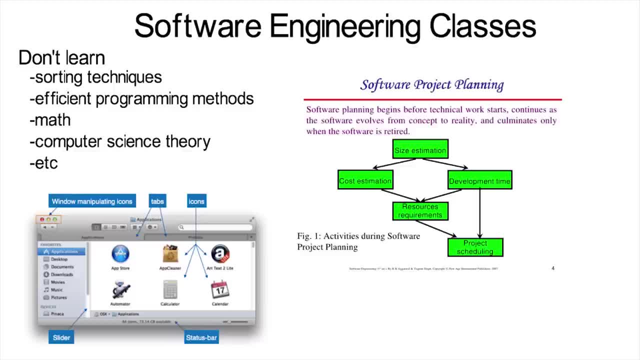 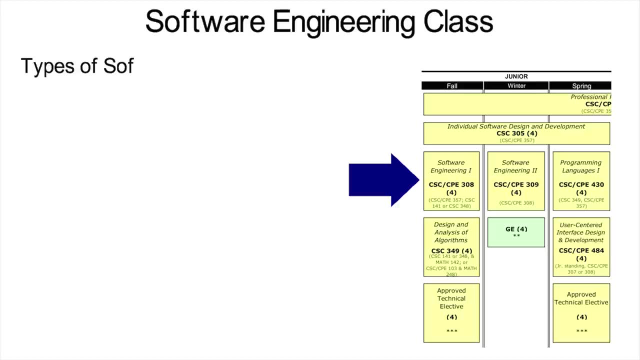 design interfaces based on who will be using your project, and so on. for example, let's look at that first class called software engineering that students at my school took their third year. students might start off by learning the types of software, such as end user, where it's used by. 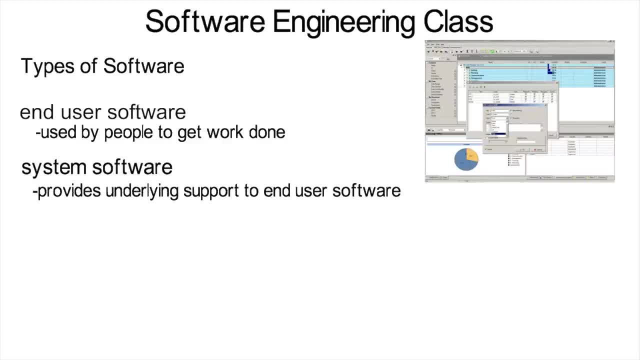 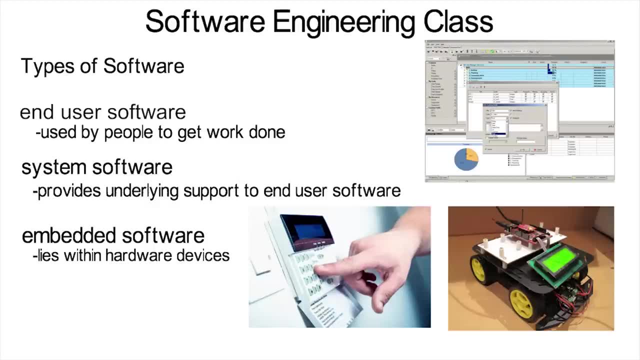 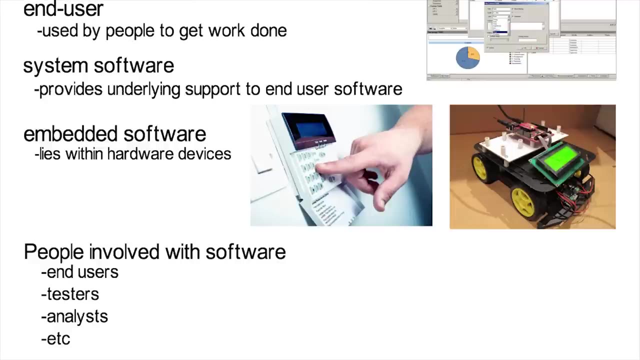 people to get work done, system software that provides underlying support to end user software, and embedded software that is within hardware devices like robots, security systems or cars. then you might define people involved with software, whether it be end users, testers, analysts, etc. as you can see, it can start off with a lot of definitions. 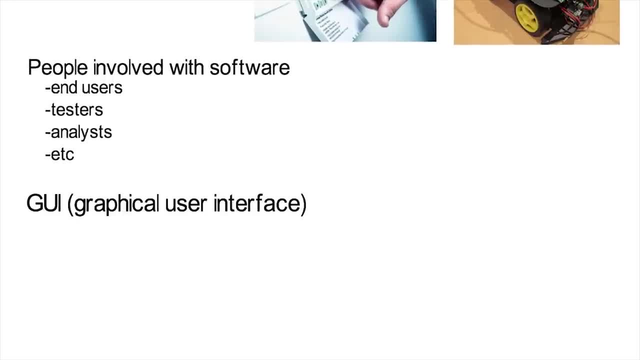 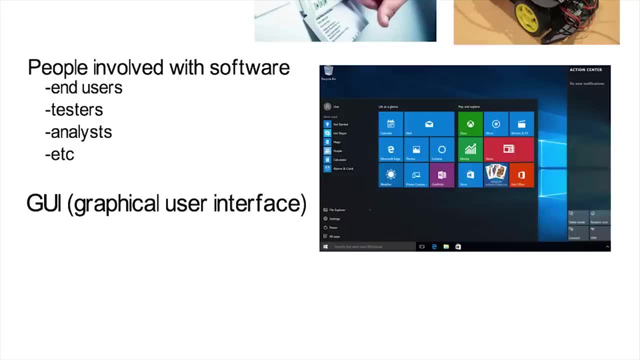 then you get into more of the software design, like prototyping a gui or graphical user interface, a way for someone to easily interact with software through graphical icons. i actually had to do this at my job before, where previous to making the gui- in order to input data into my program for 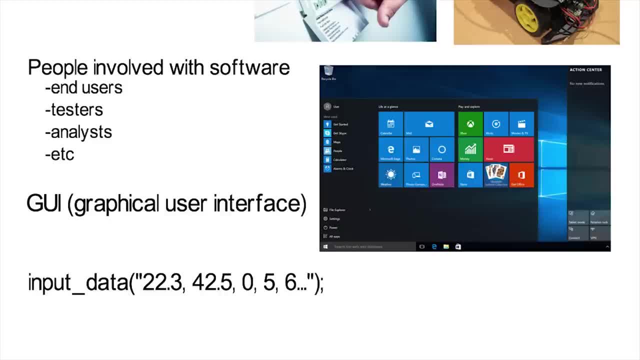 calculation. i had to type in an input command, and if i hand that code off to someone it might be annoying for them to have to figure out. so the gui instead just had a box for input values here that could easily be typed in. then, for this class, an actual exam question from a previous year when 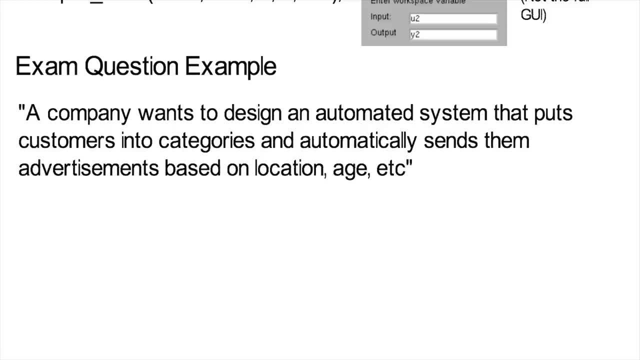 something like a company wants to design an automated system that puts customers into certain categories and automatically sends them advertisements based on location, age or whatever, and the first question was just to define a gui with file and edit menus. that would be easy to use and navigate. no coding required, though, but then you could be asked to write a java. 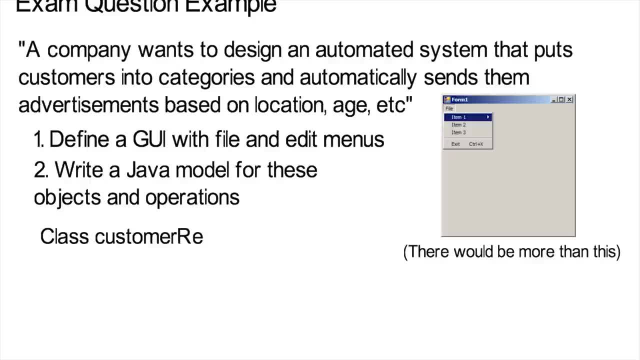 model for certain objects and operations. you'd have a class called customer records, which would need to be divided into first, middle and last name, street address and so on. you aren't writing elaborate and efficient code to actually make this system, at least on this exam question, and you're. 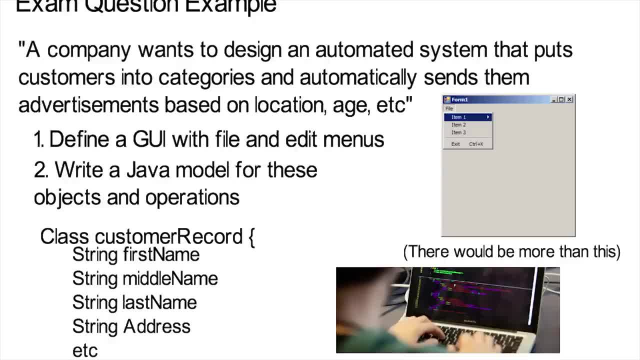 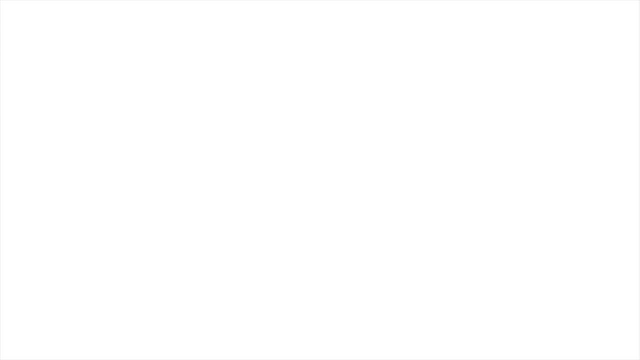 not finding a faster way to organize this list that's safe for your other classes that computer scientists also take? you're kind of planning out how the software development will happen, what things need to be taken into account, and all of that. then another class unique to software. 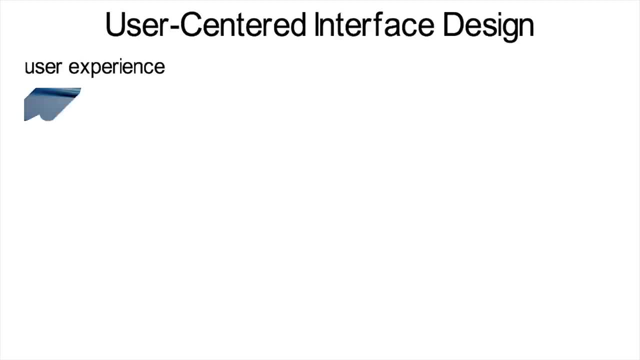 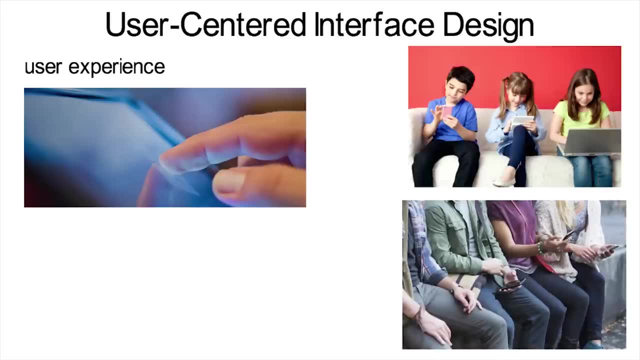 engineers is user-centered interface design. this is a class more geared towards user experience. when you make something like software for someone, you need to think about who will be using it, like children, adults, students, other engineers and so on. maybe your code should not be the most efficient if that means it's easier to use for the person. 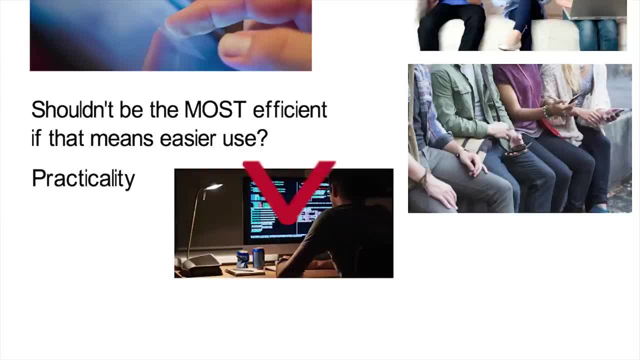 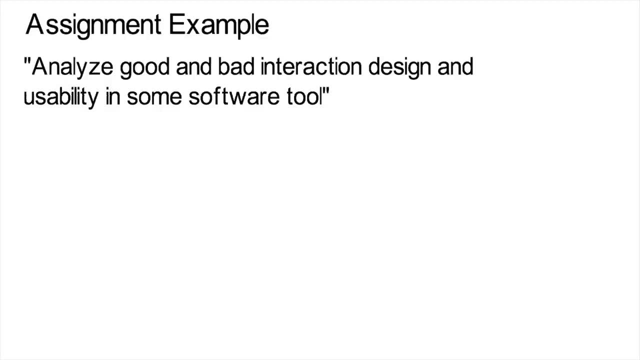 it comes down to practicality now. at my school, this class involved pretty much no programming. as an example of an assignment, you might have to analyze good and bad interaction design as well as usability in some software tool. this could be like looking at some calendar and scheduling tool and 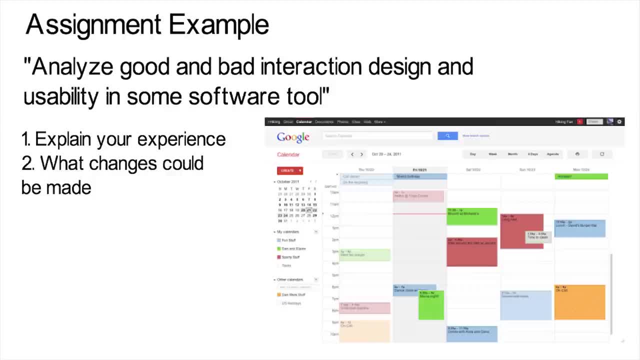 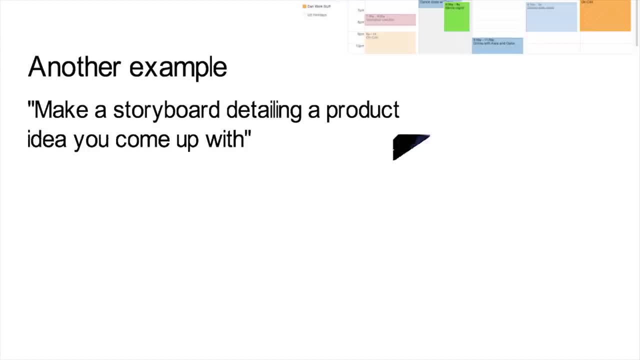 writing about your experience as a user, what changes or additions could be made for a better user experience, and so on. then you could be assigned to make a storyboard detailing a product idea you come up with, such as maybe an app that helps college students with productivity, but you wouldn't code it, or 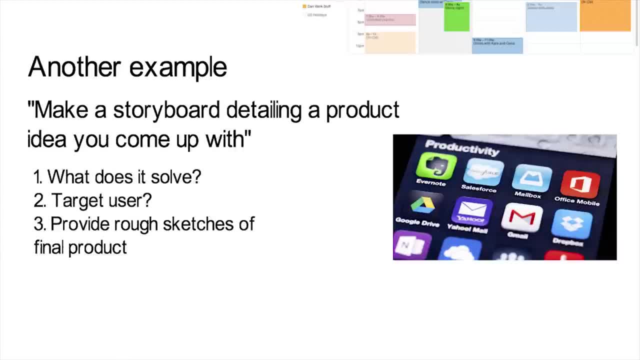 anything like that in this class. you would explain what problem it solves, who your target user is, possibly provide some rough sketches what the product would look like and more. yes, this was an actual assignment from this class. it's true, some of these classes are more on the planning side. 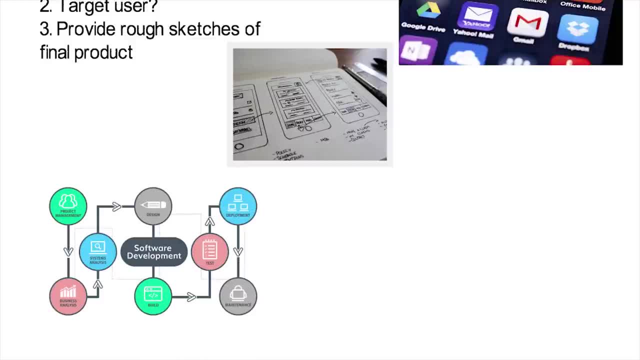 of things, rather than the real coding and development you might want to do, but these simulate what a real world project will be like when you go out and look at the class you're going to be out into your career. this will help you be prepared to work in a team and stay organized. 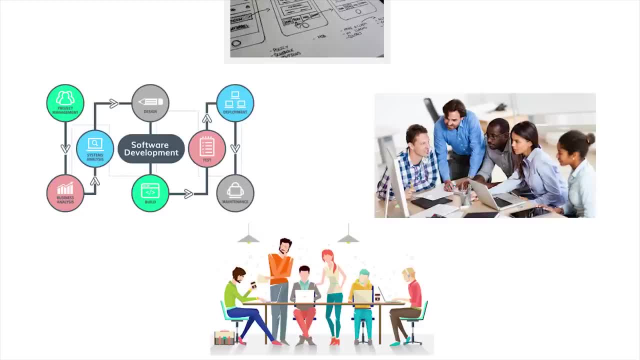 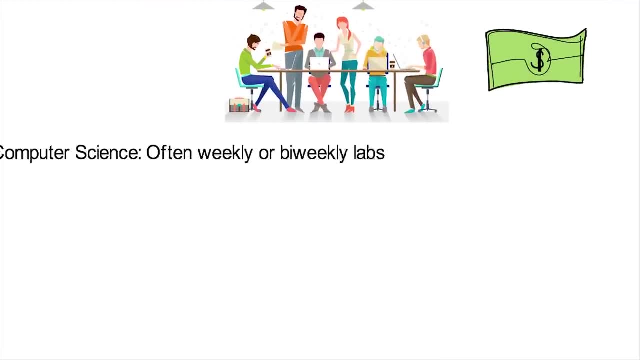 when working towards your goal. In many company settings there can be disorganization when creating a large software system, causing delays, extra costs etc. You'll also notice that in computer science classes you often do weekly or bi-weekly labs to get as much. 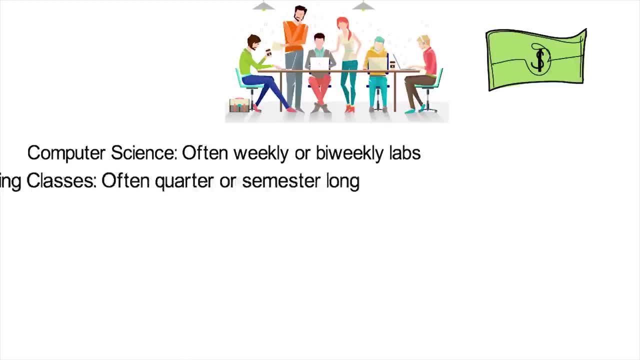 hands-on experience to go along with the theory you learn in the class. In software engineering classes it's normally quarter or semester-long projects that again simulate a real-world setting. Now, in the last few minutes, let's briefly go over courses unique to computer. 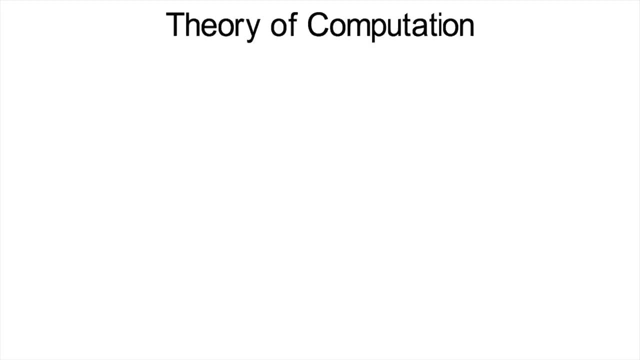 science majors, the first big one being Theory of Computation. This is, of course, a theory-heavy class that does involve math and proofs. This class won't help you write better code, but will help you understand how computer science has been thought of as a science. The big 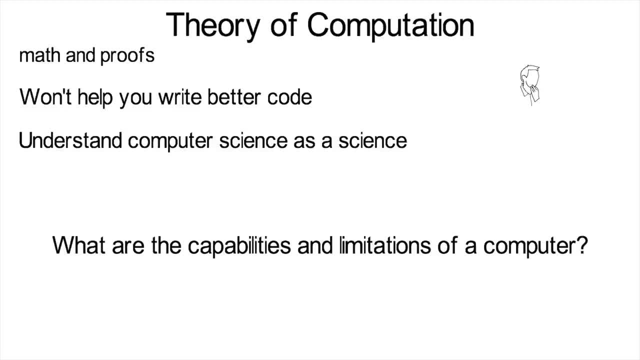 question in this class is: what are the capabilities and limitations of a computer? It's a more abstract idea Now. I've talked about this class before in other videos, but I want to do an entirely different example to not be repetitive. We're about to talk about the 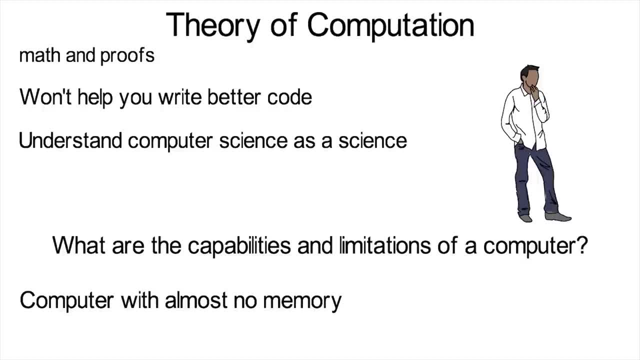 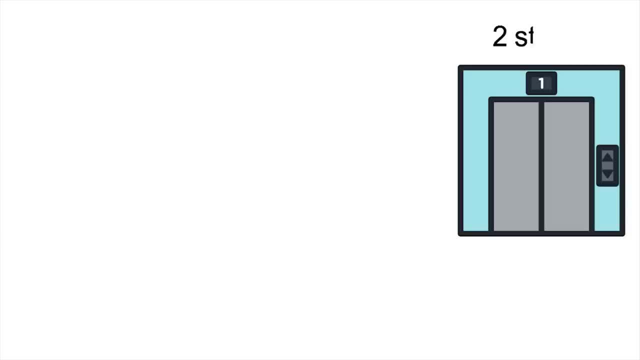 first-of-a-kind computer. We're about to see one capability of a computer with almost no memory. This is something you can expect, maybe in your first week, but we need a little background first. Let's say there's an elevator in a building with only two stories. Therefore, 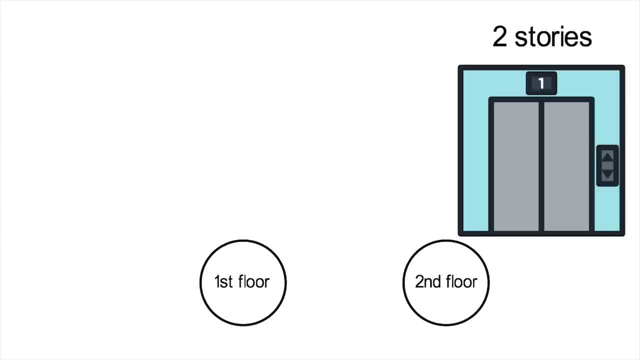 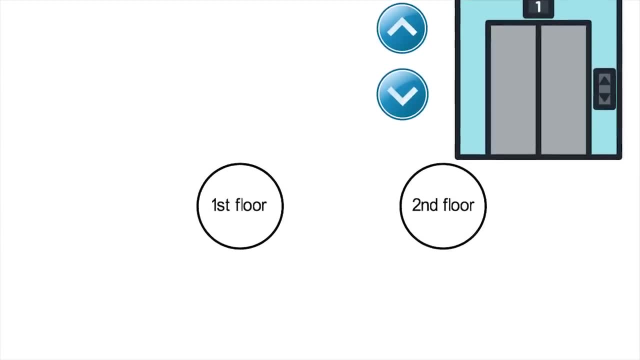 the elevator can be on the first floor or the second floor. Also, the elevator would have only two buttons on the left and right. We don't need to specify which floor. Now, if we're on the first floor and want to go to the second floor, we press the Up button. If we then want to go back down to the first floor, we press the Down button. Now we have a single elevator and it only needs two floors. For eastern systems, we have one elevator, a second floor and a second and a third floor. If we then want to go up and down, we have two floors- We press the down button. 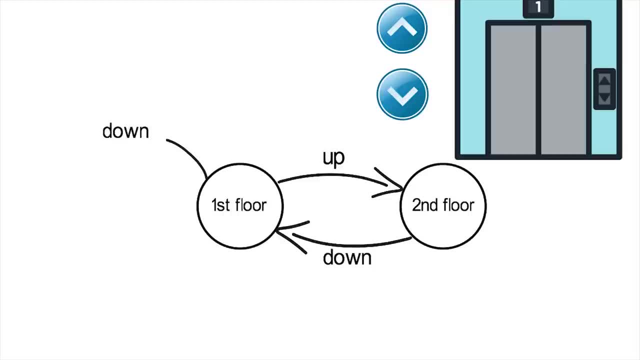 then if we're on the first floor and press down, well, we don't go anywhere, we just stay put. and if we're on the second floor and press up, the same thing happens. these things that are circled are the states of the system and these arrows are the transitions. if we replace the first and second, 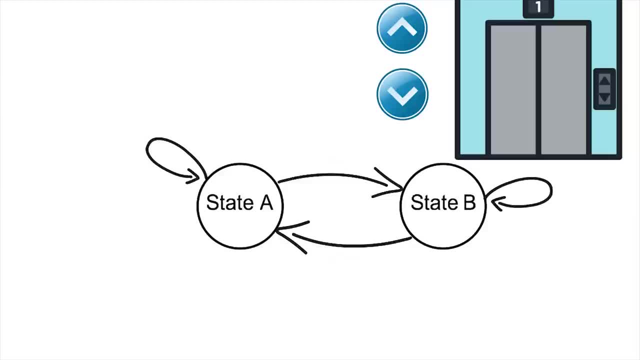 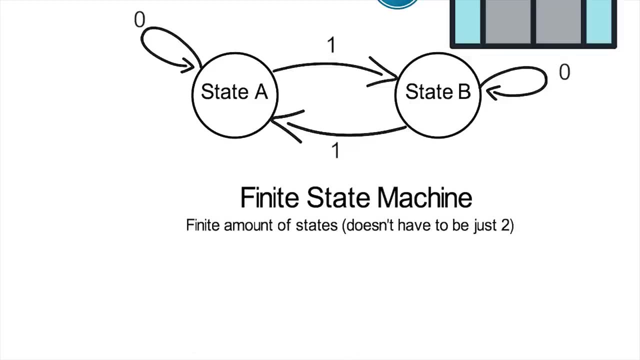 floor with general names like state a and state B, and the transitions with ones and zeros, the typical inputs and outputs for these things. we have a general finite state machine, something with, of course, a finite amount of states where the machine can change between them based on external inputs. they have very limited memory, as in. they just know which state they are in, like. 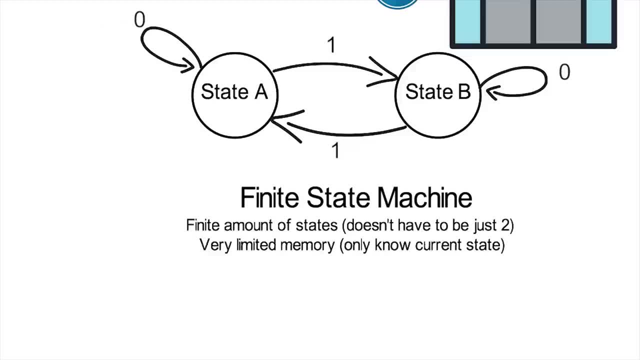 first floor or second floor, but it can't keep track of, like, how many times it went up and down. I know this is kind of abstract, but just stay with me. now here's the more interesting question. given a random list of ones and zeros, could you make one of these state machines to determine if there's 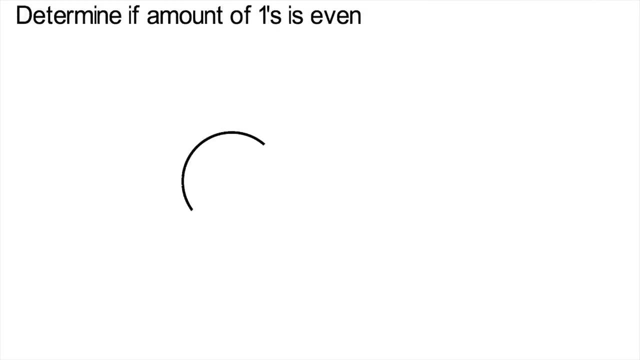 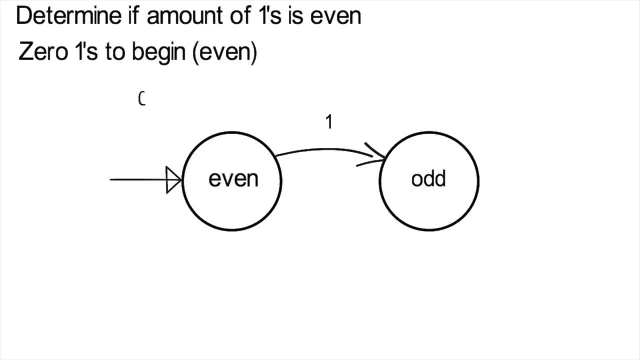 comes in, you transition to the odd state. if a zero had come first instead, there would still be an even number of ones, and if you're in the odd state and another one comes up, you transition back to even- as there have now been two ones that showed up, an even number and, of course, if the zero shows, 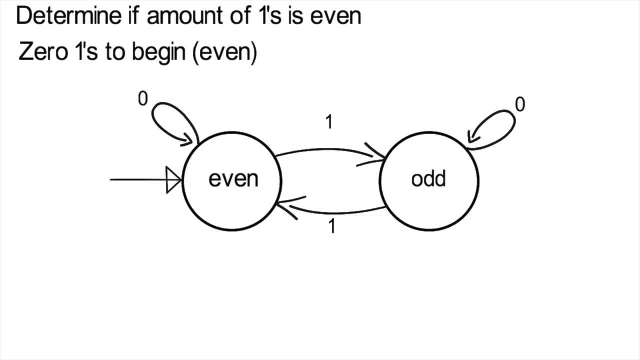 up, while in the odd state nothing happens there either. so we start at zero ones, an even number. if a one comes in, we change states to odd. if a zero then comes in, we stay in place and no matter what happens, we will always be in the proper state. remember I said this class is about the 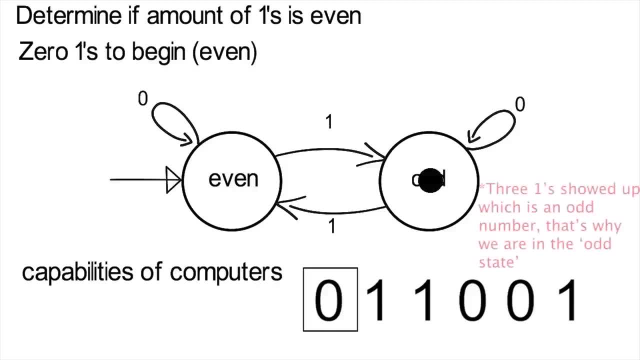 capabilities of computers. well, this hypothetical system with almost no memory is capable of determining whether there's an even or odd amount of ones in as long a list as we give it. it doesn't even have to remember the list, but if we wanted to count how many ones showed. 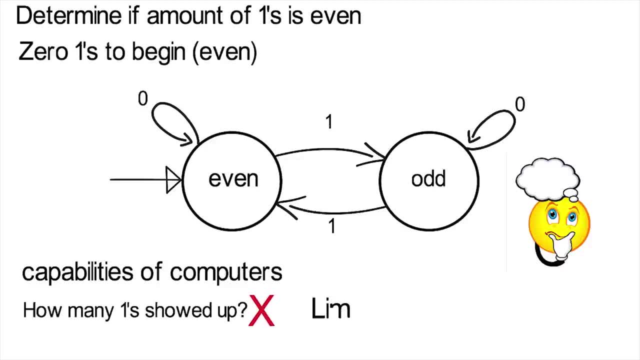 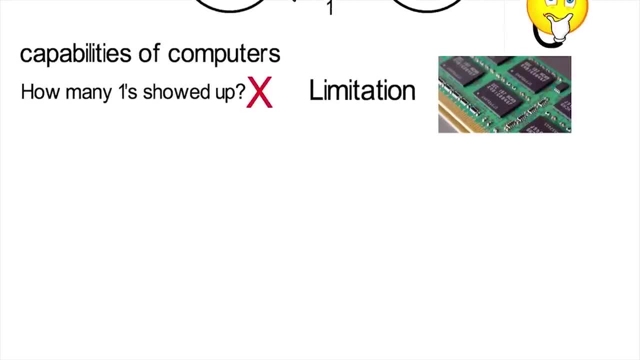 up. we couldn't do that here, at least with this setup. that's a limitation for this type of machine. and you may be thinking: well, computers do have memory, and lots of it. well, why don't we take it to another extreme? what if we had infinite memory capacity? now what? 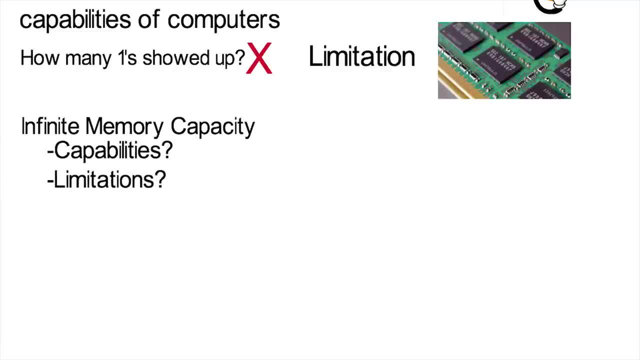 are our capabilities? what about limitations? you'll analyze this when you learn about Turing machines, an abstract machine that has an infinite memory tape to store data. if you accidentally made a program that ran forever, could this machine figure that out? well, this is the example I always use and the answer is no. you'll see that proof and more in this class. 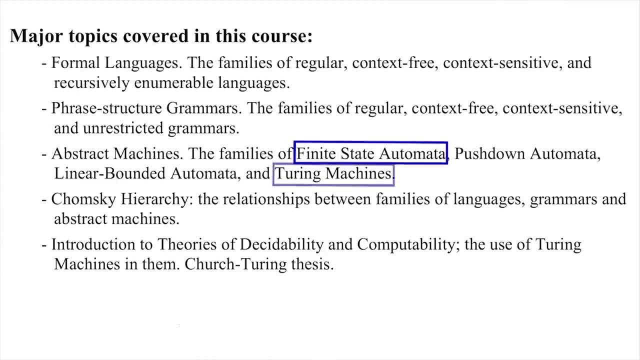 as you can see on a previous syllabus. these are just some of the things you'll learn. yes, it is theory based and abstract, but you'll think about computer science in a different way and that's the real big class that computer scientists at my school were the only ones. 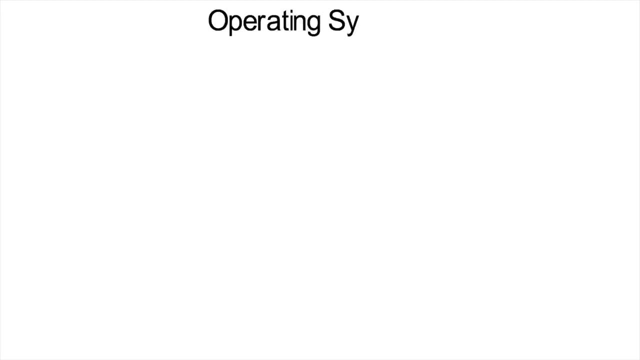 required to take. another one, though, that software engineers don't take is operating systems, which is the software that supports a computer's functions, such as executing various applications and scheduling what tasks to do. Microsoft, Windows and iOS are operating systems and, as you probably know, these are constantly updated by engineers. 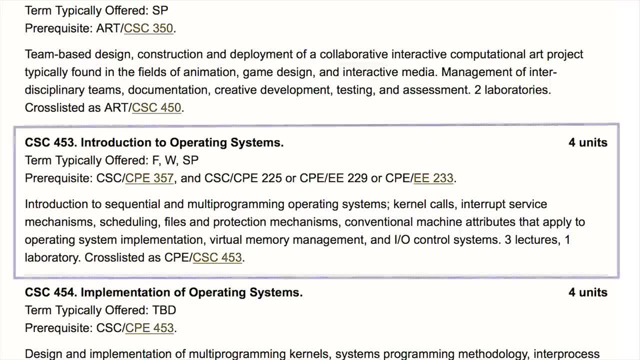 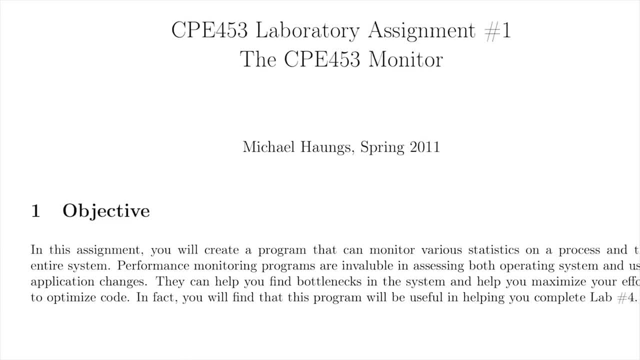 fixed for bugs and so on. this class is pretty technical, which you can see by its description and on a syllabus. you see it contains plenty of labs, which again is common for computer science classes. and that's about it for the differences I'll go over because, remember, these majors are: 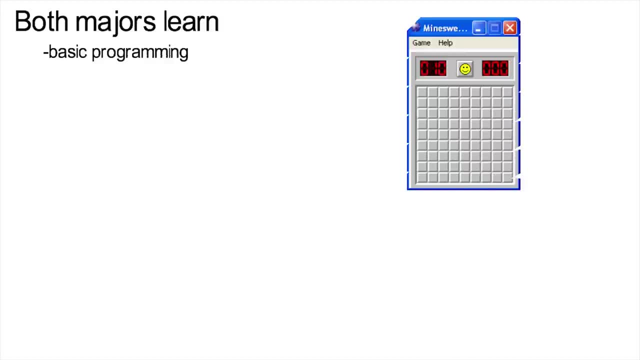 mostly the same. both will learn the basics of programming and will make simple games. they'll both learn data structures and how to store an array of numbers and sort it quickly. both take discrete math and learn proof techniques, set theory etc. then apply it to your algorithms class to find, like, the shortest distance from one point to another.